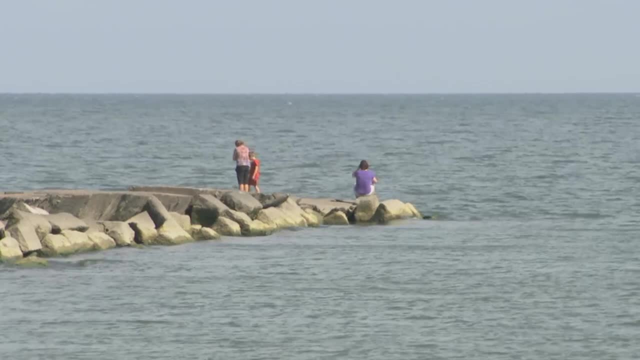 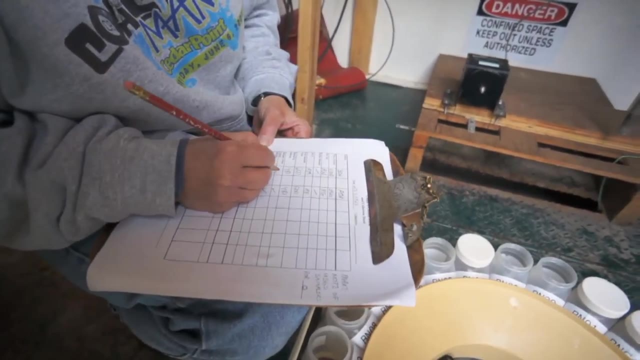 After that, phosphates were banned in laundry detergent, Phosphorus was reduced and things got better. But in recent years algal blooms have been making a comeback and Heidelberg researchers think they've found out why It's called dissolved phosphorus. 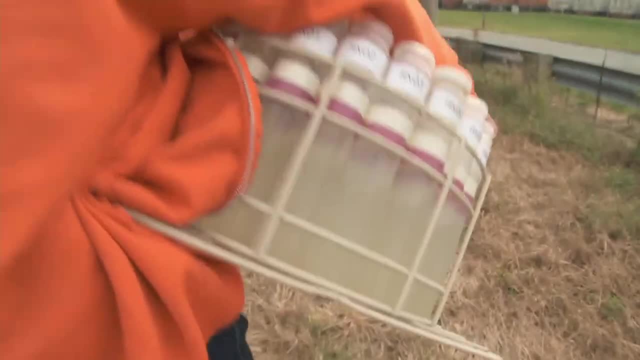 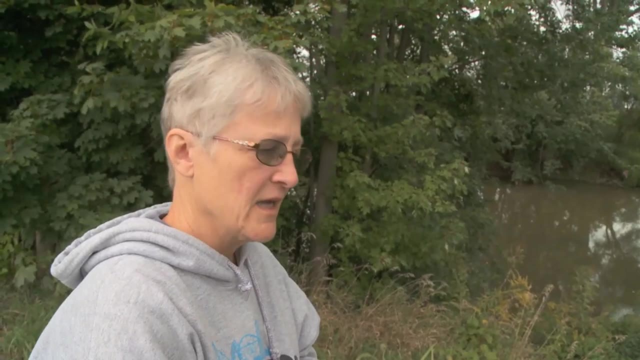 It's said, dissolved phosphorus was like a power bar for the toxic algae. If you were to ask five years ago dissolved phosphorus, everybody would scratch their head and go what's that? And they now feel that that's really the component, one of the main components. 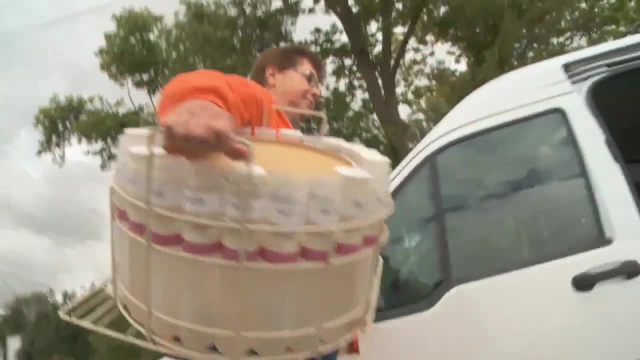 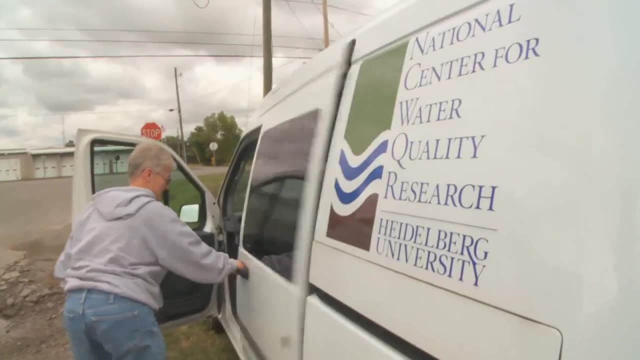 in contributing to the algal bloom. We like to think that we know everything that's going on out here, but sometimes it takes a little bit longer term of sampling and database and data analysis to really start to see trends, Though there are several sources of dissolved phosphorus in Lake Erie, 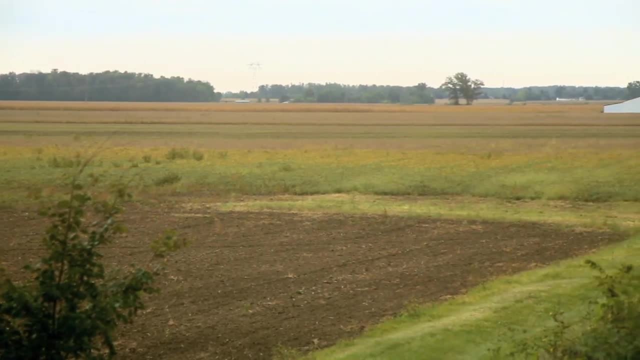 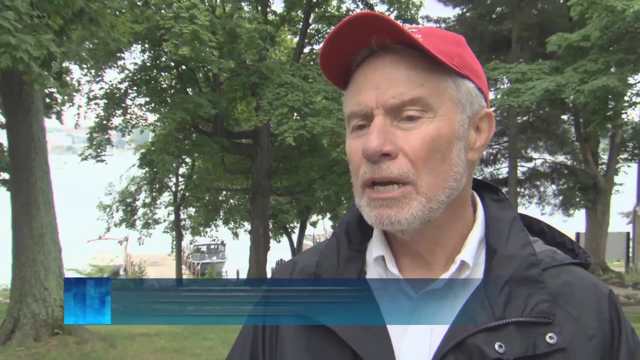 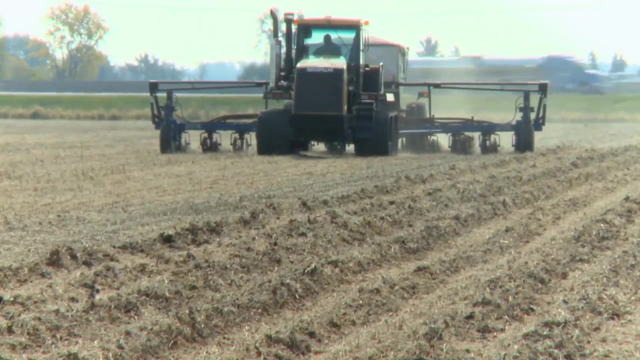 scientists believe most of the problem comes from farm fertilizer. The other ones all contribute, but the one that contributes the most, or puts in the largest portion of the load, is agricultural runoff, And so we're trying to get farmers to not apply more than they need and modify the way that they apply the fertilizer. 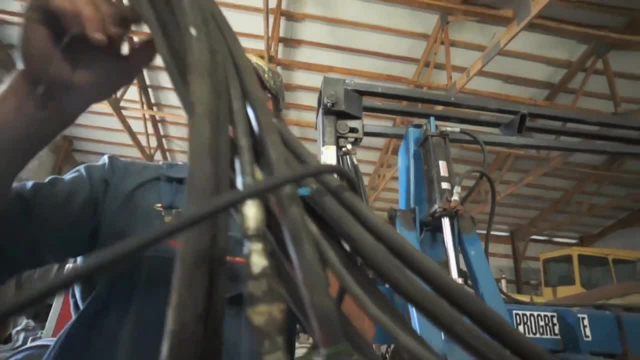 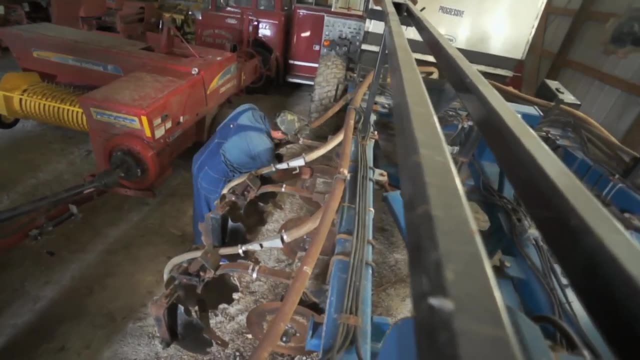 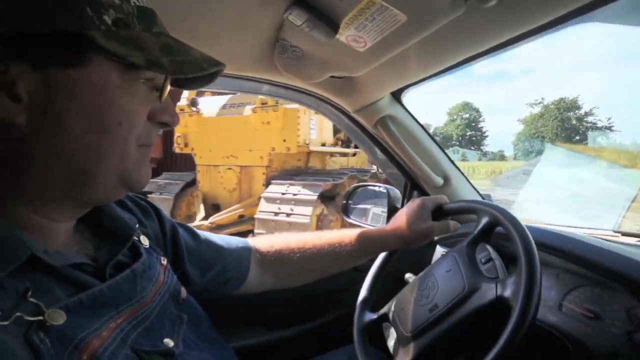 And we think that pretty much those two things together will solve the problem. This year, the Ohio Farm Bureau began promoting ways to better apply fertilizer, using the right amount at the right time. This farm has been in the family since 1890.. The Myers farm is near Toledo, less than a mile from Lake Erie. 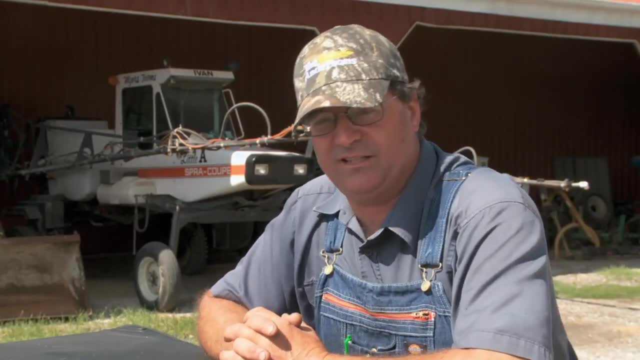 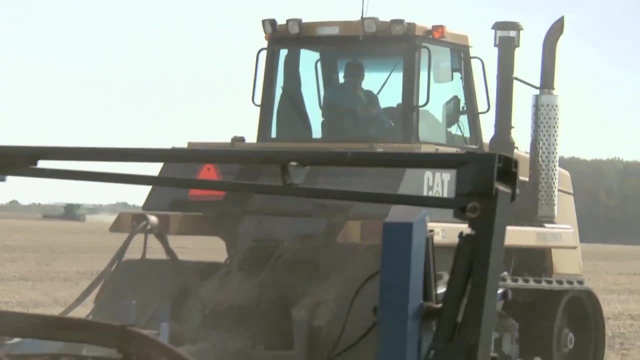 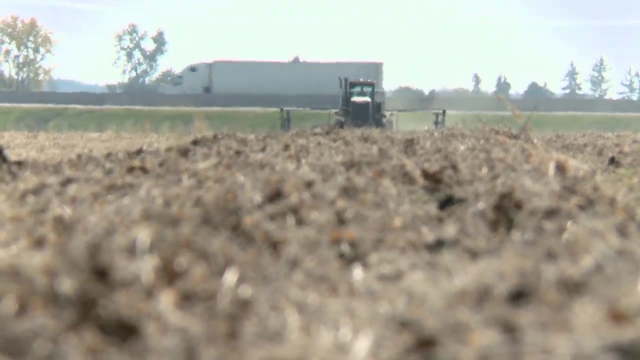 My great-grandfather is the one that first started this. My son's the fifth generation, Bill Myers, says he's been applying fertilizer the way the Farm Bureau recommends for years. It's just common sense, really. It bothers him that farmers are so often blamed for the algal blooms. 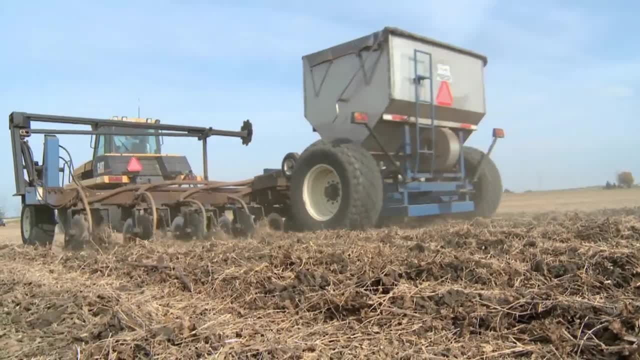 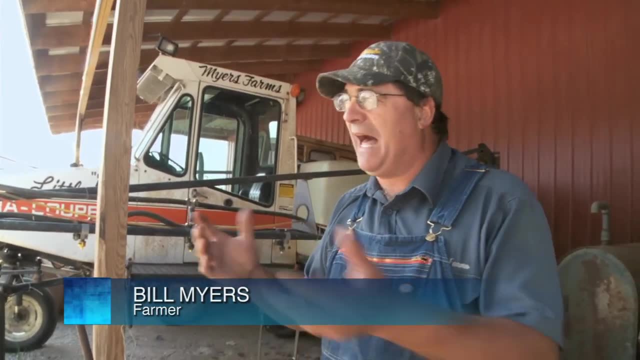 The people that will listen to these interviews or read the articles in the paper. the point they don't understand is: there isn't some great big pile of phosphorus someplace that the government gives us for free, that they don't want to use. 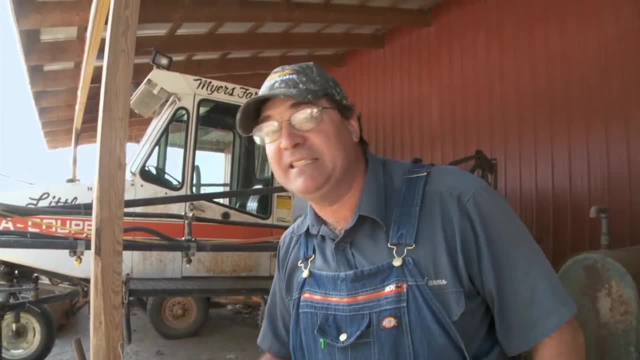 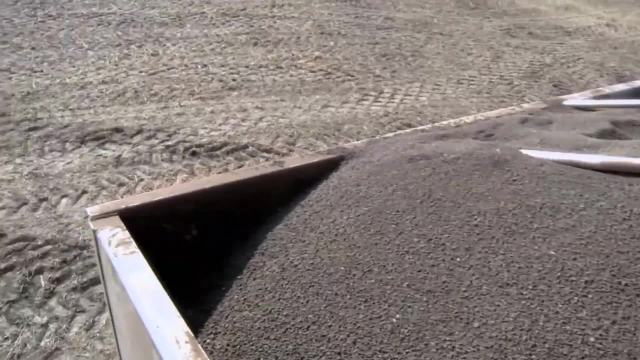 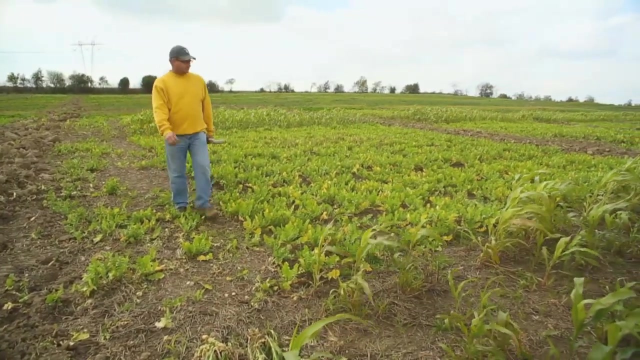 They say, hey, use all you want, It's expensive. It costs hundreds of dollars an acre to purchase and apply Best agricultural practices that reduce harmful runoff can be expensive. That's why programs like this one that help farmers grow cover crops in the fall are so important.